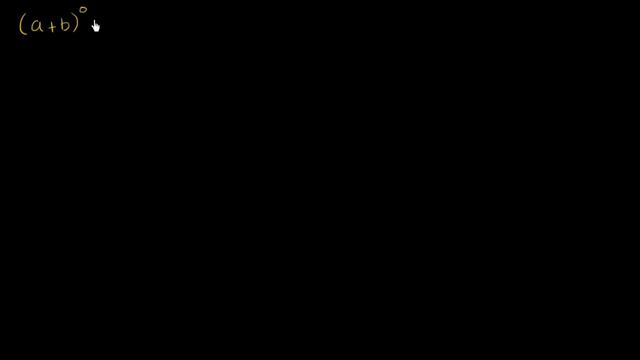 Let's take that to the zero power. Well, anything that's non-zero, to the zero power, that's just going to be equal to 1.. Well, that wasn't too bad. Now, what about a plus b to the first power? 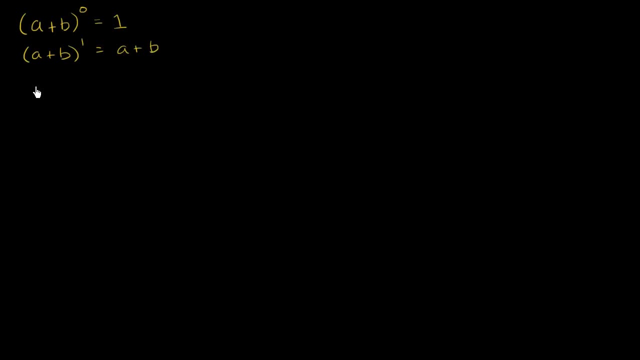 Well, that's just going to be a plus b. Now. what about a plus b squared? Now, if you haven't been practicing taking powers of binomials, you might have been tempted to say a squared plus b squared, But that would be incorrect. 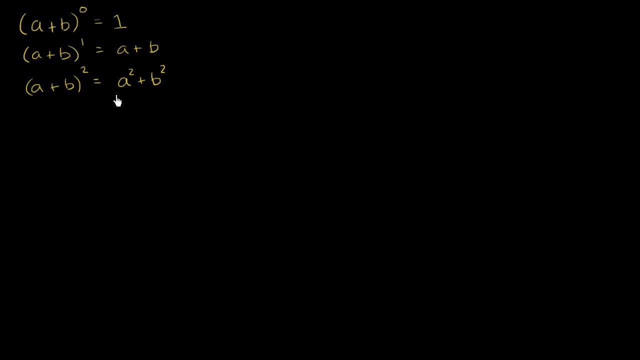 If you did that, you should give yourself a very gentle but not overly discouraging slap on the wrist or the brain or something. a plus b squared is not a squared plus b squared. It is a plus b times a plus b. And then, if you do this, it'll be a times a, which is a squared. 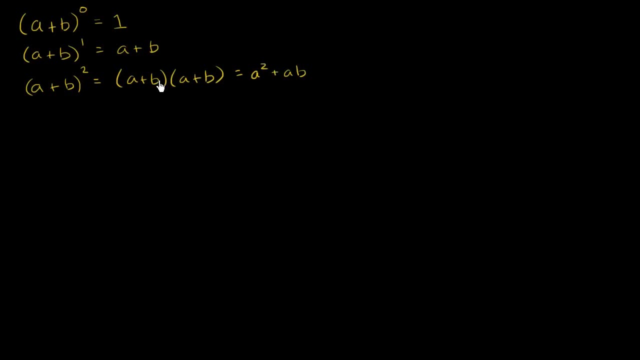 plus a times b, which is ab, plus b times a, which is another ab plus b times b, which is b squared. You have two ab's here, so you could add them together, So it's equal to a squared plus 2ab plus b squared. 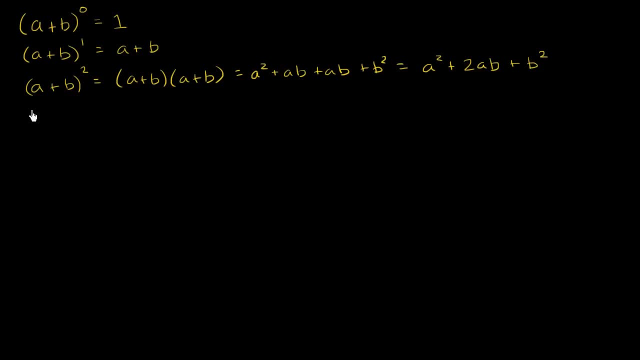 Now things are going to get a little bit more interesting. What is a plus b to the third power going to be equal to? And I encourage you to pause this video and try to figure that out on your own. Well, we know that a plus b to the third power is just a plus b to the second power, times another a plus b. 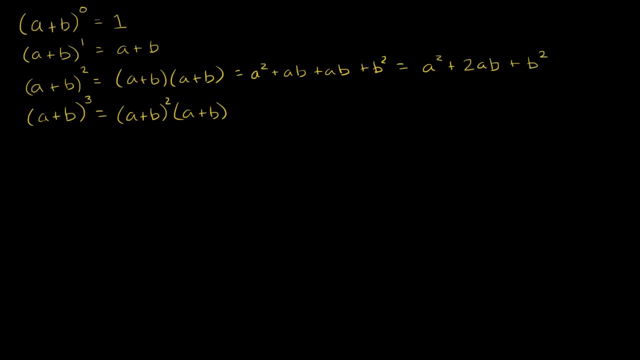 So let's just multiply this times a plus b to figure out what it is. And I'll do this. So let's see, Let's multiply that times a plus b. So I'm just going to multiply it this way. So first I'll multiply b times all of these things. 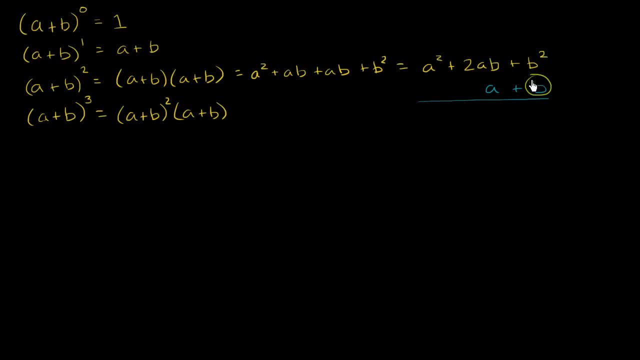 So I'll do it in this green color: b times b squared is b to the third power. b times 2ab is 2ab squared, So 2ab squared. And then b times a squared is ba squared or a squared b. 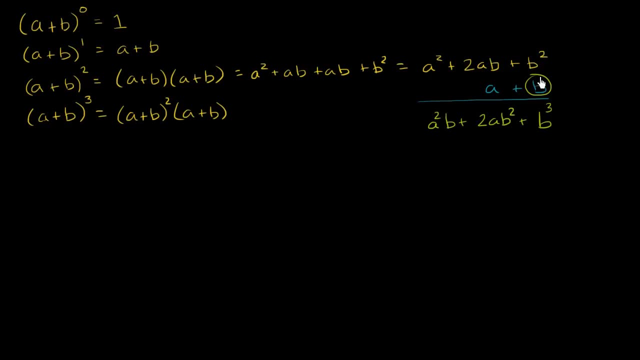 a squared b. So all I did is I multiplied b times all of this stuff. Now let's multiply a times all of this stuff. a times b squared is ab squared. ab. squared a times 2ab is 2a squared b. 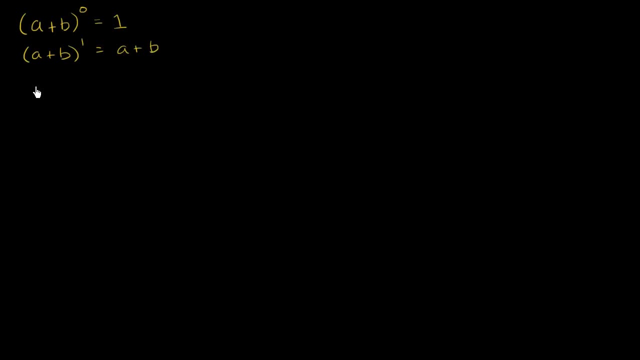 Well, that's just going to be a plus b. Now. what about a plus b squared? Now, if you haven't been practicing taking powers of binomials, you might have been tempted to say a squared plus b squared, But that would be incorrect. 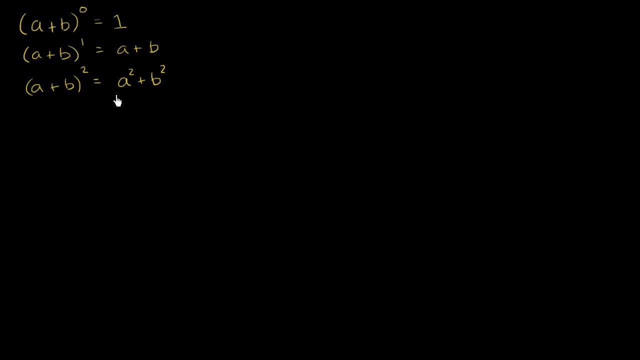 If you did that, you should give yourself a very gentle but not overly discouraging slap on the wrist or the brain or something. a plus b squared is not a squared plus b squared. It is a plus b times a plus b. And then, if you do this, it'll be a times a, which is a squared. 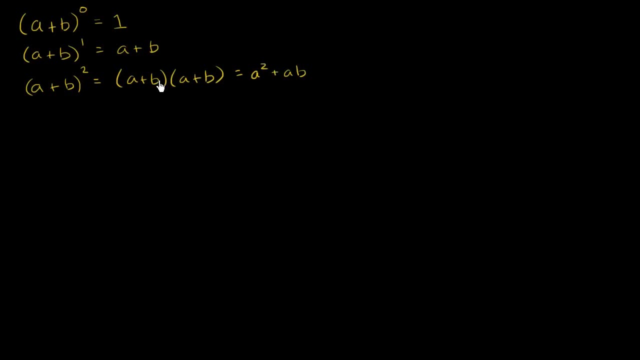 plus a times b, which is ab, plus b times a, which is another ab plus b times b, which is b squared. You have two ab's here, so you could add them together, So it's equal to a squared plus 2ab plus b squared. 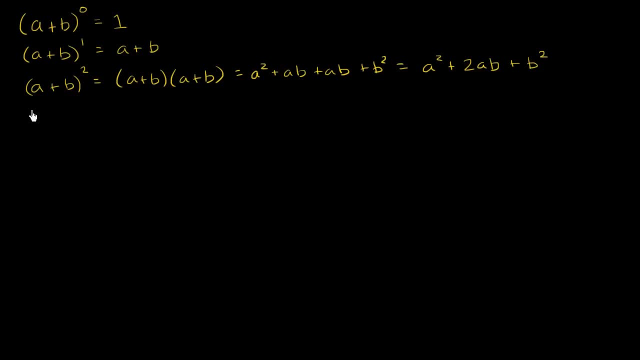 Now things are going to get a little bit more interesting. What is a plus b to the third power going to be equal to? And I encourage you to pause this video and try to figure that out on your own. Well, we know that a plus b to the third power is just a plus b to the second power, times another a plus b. 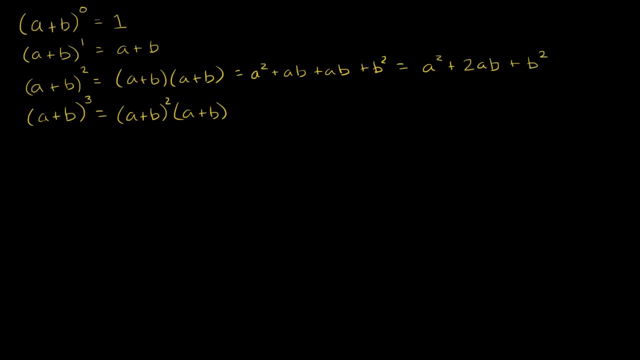 So let's just multiply this times a plus b to figure out what it is. And I'll do this. So let's see, Let's multiply that times a plus b. So I'm just going to multiply it this way. So first I'll multiply b times all of these things. 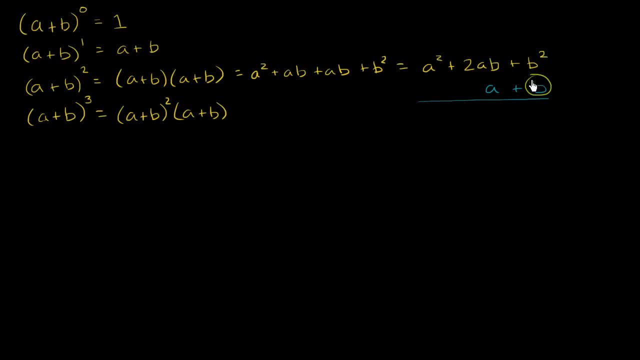 So I'll do it in this green color: b times b squared is b to the third power. b times 2ab is 2ab squared, So 2ab squared. And then b times a squared is ba squared or a squared b. 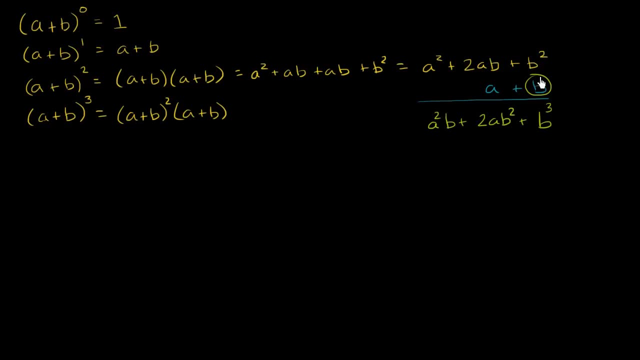 a squared b. So all I did is I multiplied b times all of this stuff. Now let's multiply a times all of this stuff. a times b squared is ab squared. ab. squared a times 2ab is 2a squared b. 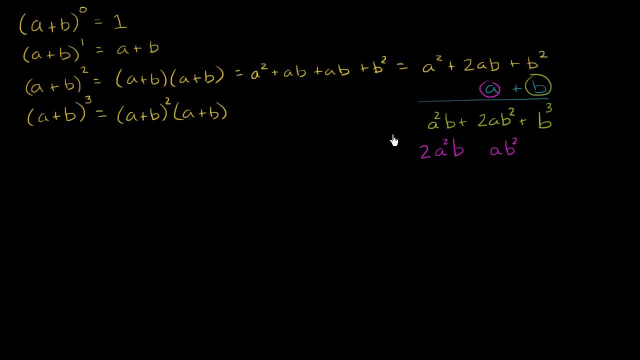 2a squared b And then a times a squared is a to the third power. And now when we add all of these things together, we get a to the third power, plus let's see we have one a squared b plus two more a squared b's. 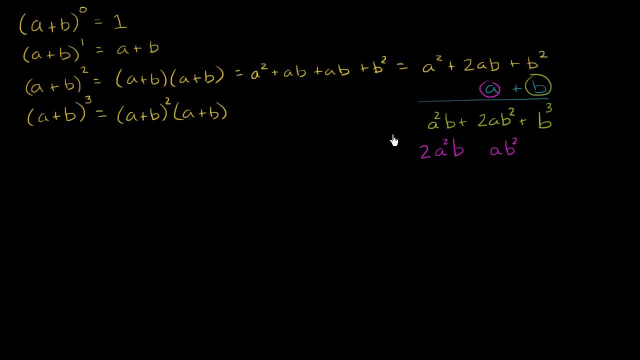 2a squared b And then a times a squared is a to the third power. And now when we add all of these things together, we get a to the third power, plus let's see we have one a squared b plus two more a squared b's. 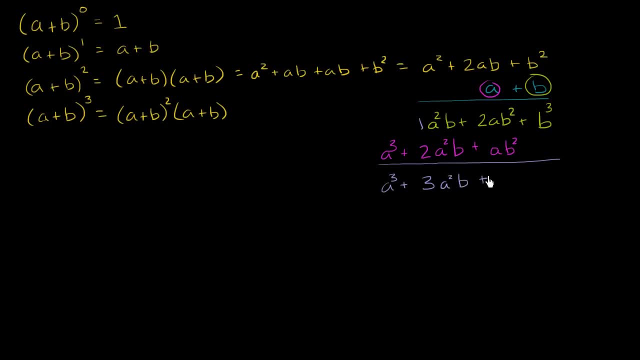 That's going to be 3a squared b Plus 3ab squared, 2ab squared plus another ab squared is going to be 3ab squared plus b to the third power. So just taking something to the third power has already took us a reasonable amount of time. 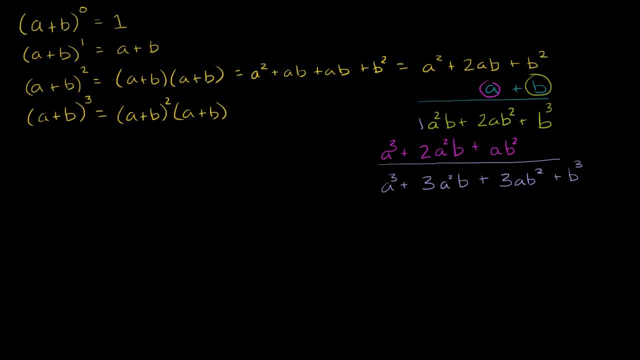 And so you can imagine how painful it might get to do something like a plus b to the fourth power. Or, even worse, if you were trying to find a plus b to the tenth power or to the twentieth power, This would take you all day, or maybe even longer than that. 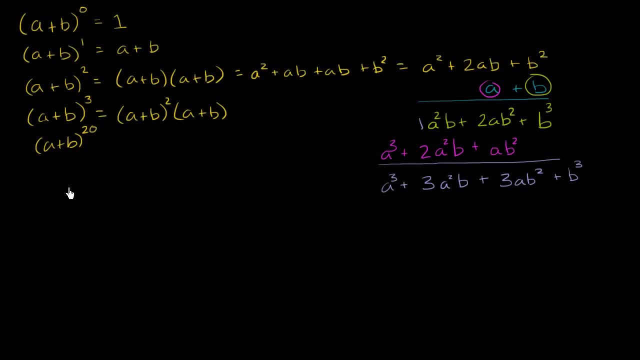 It would be incredibly, incredibly painful. And that's where the binomial theorem becomes useful. So what is the binomial theorem? Well, the binomial theorem tells us. let me write this down: Binomial theorem, Binomial theorem: It tells us that if we have a binomial 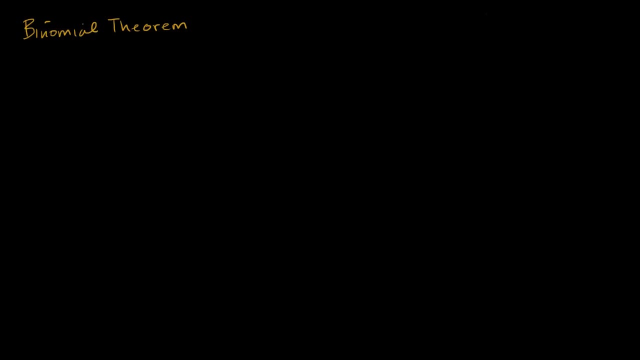 I'll just stick with the a plus b for now. if I have- and I'm going to try to color code this a little bit- if I have, the binomial a plus b, a plus b, and I'm going to raise it to the nth power. 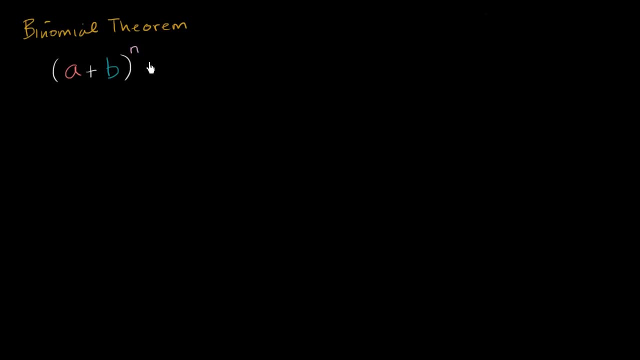 I'm going to raise this to the nth power. the binomial theorem tells us that this is going to be equal to- and the notation is going to look a little bit complicated at first, but then we'll work through an actual example- is going to be equal to: the sum from k equals 0,. 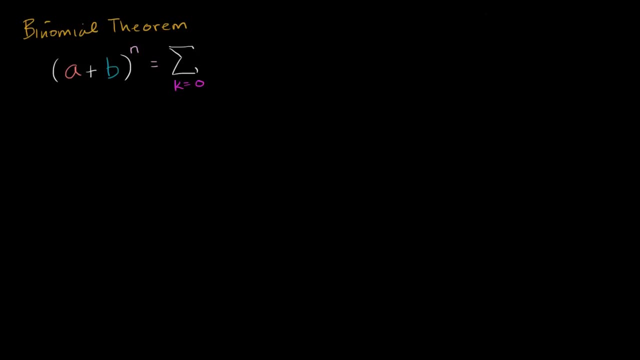 k equals 0, to n. this n and this n are the same number of. I don't want that's kind of a garish color of n, choose k, n, choose k, and we'll review that in a second. 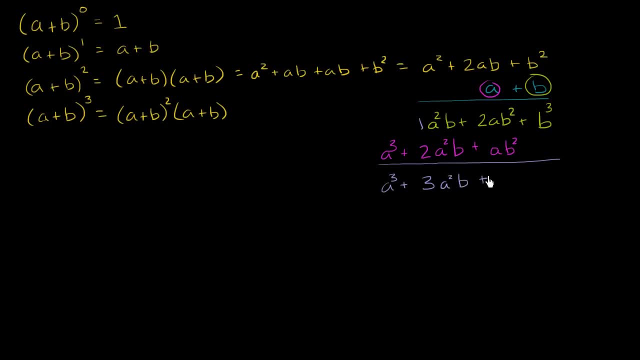 That's going to be 3a squared b Plus 3ab squared, 2ab squared plus another ab squared is going to be 3ab squared plus b to the third power. So just taking something to the third power has already took us a reasonable amount of time. 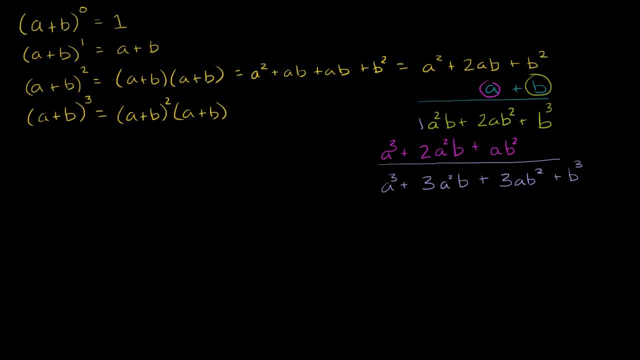 And so you can imagine how painful it might get to do something like a plus b to the fourth power. Or, even worse, if you were trying to find a plus b to the tenth power or to the twentieth power, This would take you all day, or maybe even longer than that. 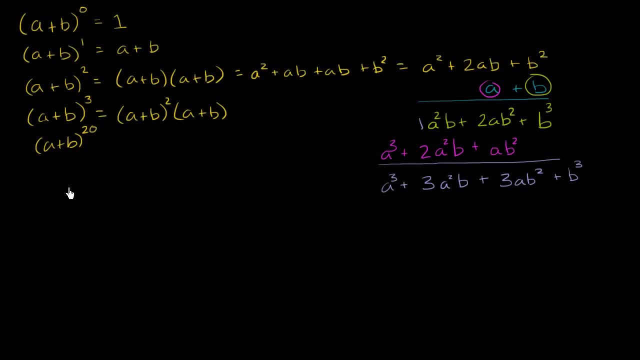 It would be incredibly, incredibly painful. And that's where the binomial theorem becomes useful. So what is the binomial theorem? Well, the binomial theorem tells us. let me write this down: Binomial theorem, Binomial theorem: It tells us that if we have a binomial 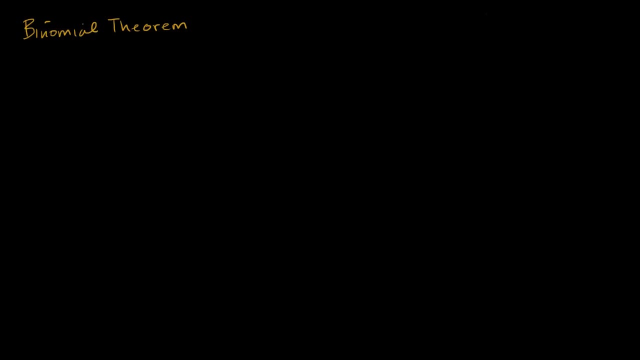 I'll just stick with the a plus b for now. if I have- and I'm going to try to color code this a little bit- if I have, the binomial a plus b, a plus b, and I'm going to raise it to the nth power. 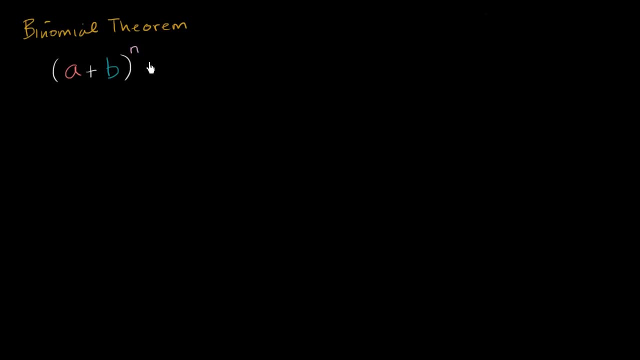 I'm going to raise this to the nth power. the binomial theorem tells us that this is going to be equal to- and the notation is going to look a little bit complicated at first, but then we'll work through an actual example- is going to be equal to: the sum from k equals 0,. 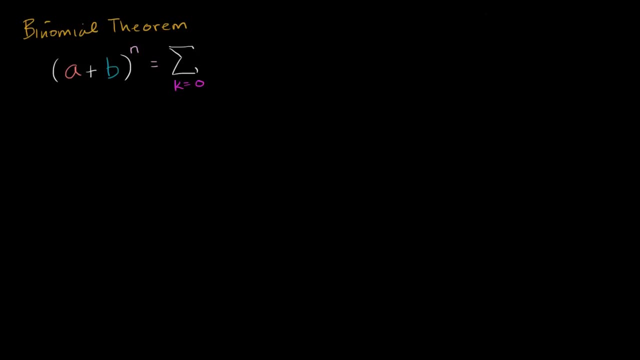 k equals 0, to n. this n and this n are the same number of. I don't want that's kind of a garish color of n, choose k, n, choose k, and we'll review that in a second. 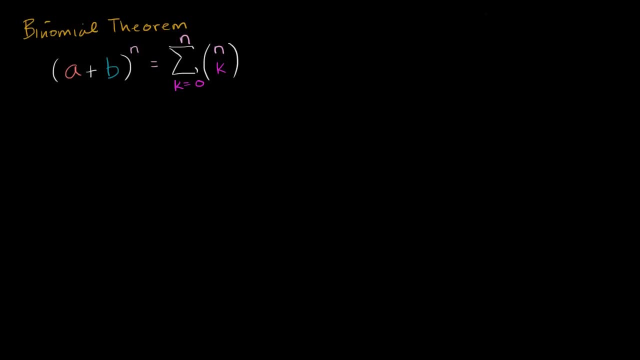 this comes straight out of combinatorics: n choose k times a to the n minus k, n minus k times b times b to the k, b to the k power. now this seems a little bit unwieldy, and let's just review, remind ourselves what n choose k actually means. 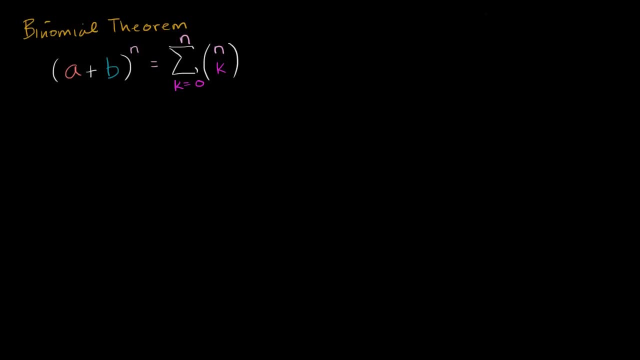 this comes straight out of combinatorics: n choose k times a to the n minus k, n minus k times b times b to the k, b to the k power. now this seems a little bit unwieldy, and let's just review, remind ourselves what n choose k actually means. 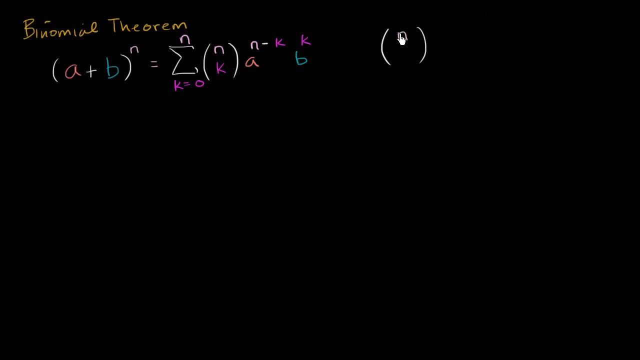 so if we say n choose k, I'm going to do the same colors, n choose k we remember from combinatorics. this would be equal to n. factorial. n. factorial over over k. factorial over k. factorial times. n minus k factorial. 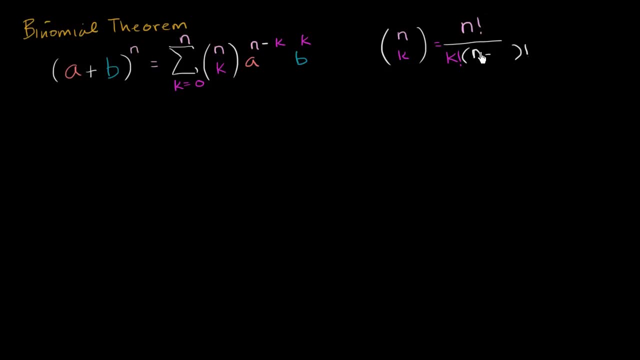 n minus k factorial, so n minus k, minus k factorial. let me color code this: n minus k factorial. so let's try to apply this and let's just start applying it to the thing that started to intimidate us. say a plus b to the fourth power. 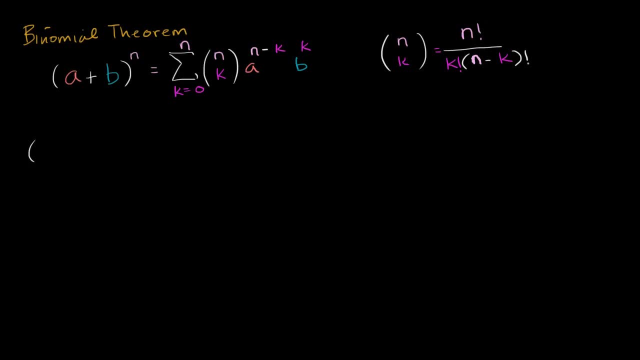 so let's figure out what that's going to be. let's try this. so: a- I'm going to try to keep it color coded so you know what's going on. a plus b, although it takes me a little bit more time to keep switching colors. 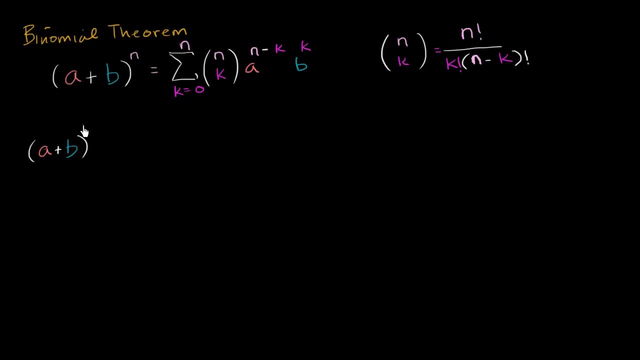 but hopefully it's worth it. a plus b. let's take that to the fourth power. so the binomial theorem tells us this is going to be equal to- and I'm just going to use this exact notation- this is going to be the sum. 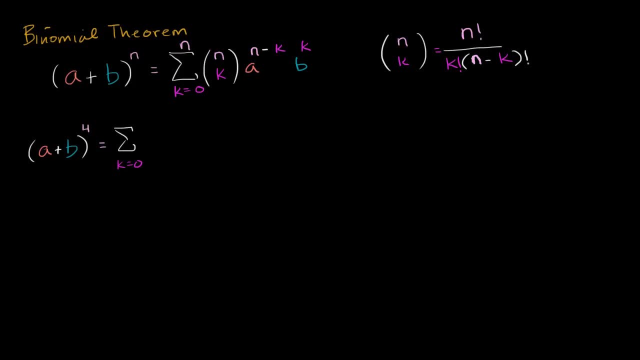 from k equals zero. k equals zero to four to four of of four. choose k four. choose k four. choose- let me do that- k in that purple color. four. choose k of a to the n or the four minus k. power. 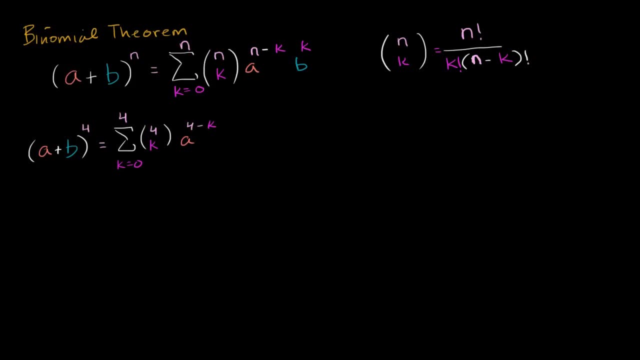 four minus k power, times b to the k power, b to the k power. now, what is that going to be equal to? Well, let's just actually just do the sum this is going to be equal to. so we're going to start at: k equals zero. 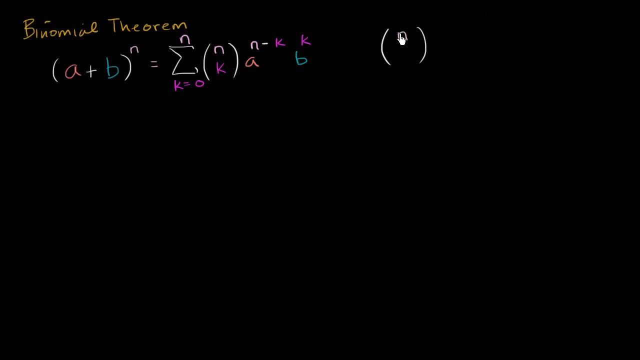 so if we say n choose k, I'm going to do the same colors, n choose k we remember from combinatorics. this would be equal to n. factorial. n. factorial over over k. factorial over k. factorial times. n minus k factorial. 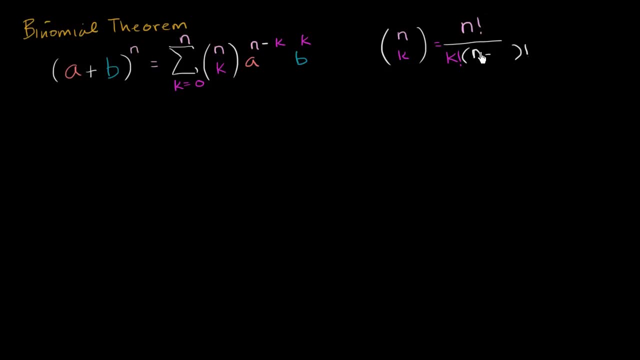 n minus k factorial, so n minus k, minus k factorial. let me color code this: n minus k factorial. so let's try to apply this and let's just start applying it to the thing that started to intimidate us. say a plus b to the fourth power. 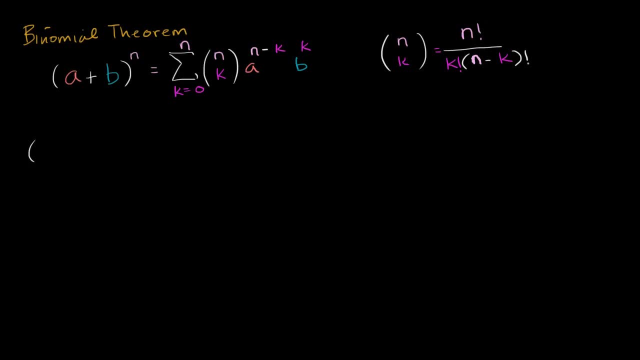 so let's figure out what that's going to be. let's try this. so: a- I'm going to try to keep it color coded so you know what's going on. a plus b, although it takes me a little bit more time to keep switching colors. 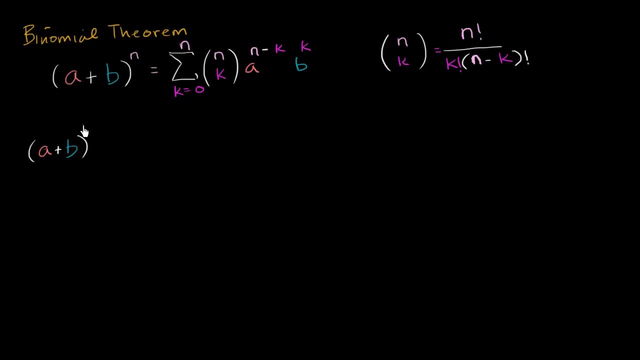 but hopefully it's worth it. a plus b. let's take that to the fourth power. so the binomial theorem tells us this is going to be equal to- and I'm just going to use this exact notation- this is going to be the sum. 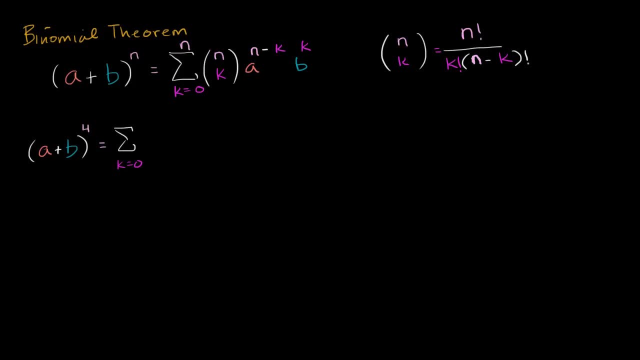 from k equals zero. k equals zero to four to four of of four. choose k four. choose k four. choose- let me do that- k in that purple color. four. choose k of a to the n or the four minus k. power. 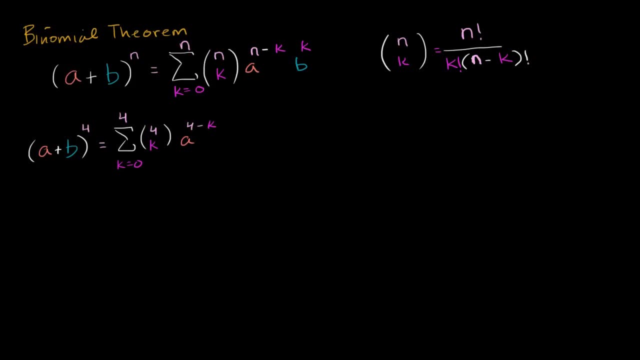 four minus k power, times b to the k power, b to the k power. now, what is that going to be equal to? Well, let's just actually just do the sum this is going to be equal to. so we're going to start at: k equals zero. 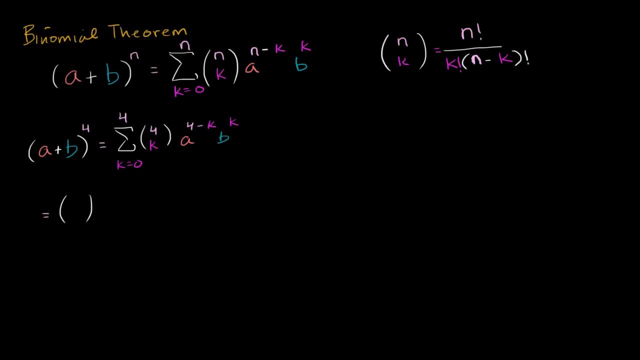 so when k equals zero, it's going to be four choose zero, four choose zero. times a to the four minus zero power. well, that's just going to be a to the fourth power, times b to the zero power. well, b to the zero power is just going to be equal to one. 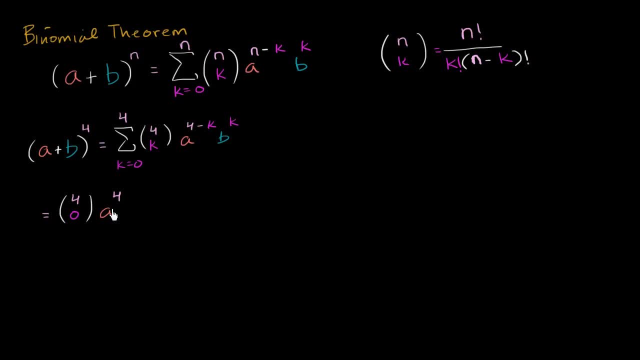 so we could just put a one here if we want to, or we could just leave it like that. so this is what we get when k equals zero, and then to that we're going to add when k equals one. so k equals one is going to be: 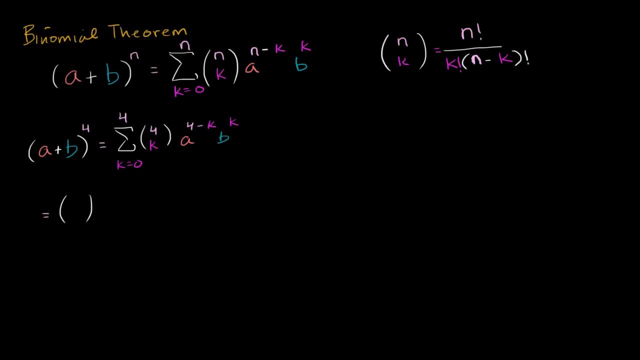 so when k equals zero, it's going to be four choose zero, four choose zero. times a to the four minus zero power. well, that's just going to be a to the fourth power, times b to the zero power. well, b to the zero power is just going to be equal to one. 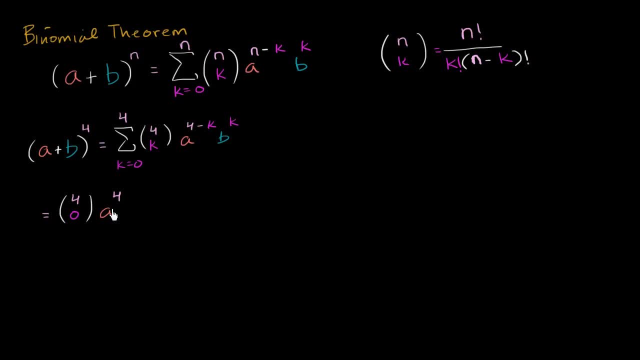 so we could just put a one here if we want to, or we could just leave it like that. so this is what we get when k equals zero, and then to that we're going to add when k equals one. so k equals one is going to be: 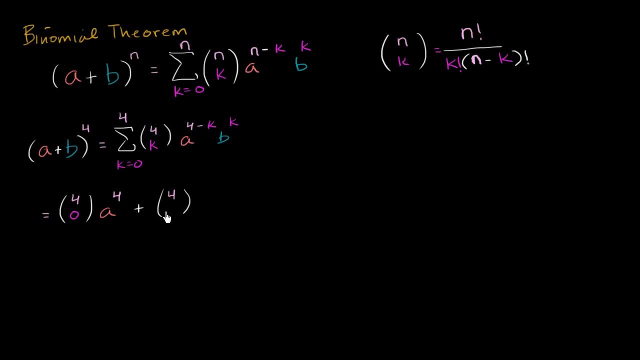 the coefficient is going to be four, choose one. and it's going to be times a to the four minus one power. so a to the third power, and I'll just stick with that color. times b to the k power. well, now, k is one. 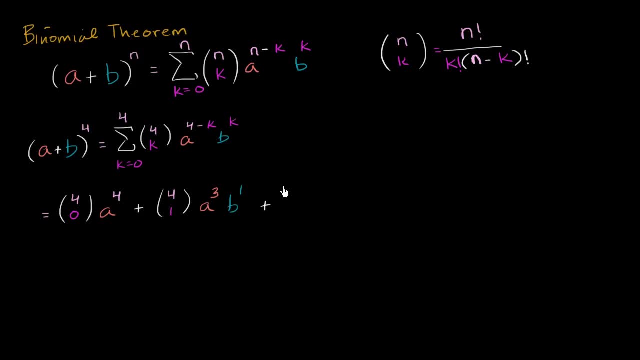 b to the first power, and then to that we're going to add, we're going to add four, choose two. four, choose two times a to the well now k is two. four minus two is two a squared. I think you see a pattern here. 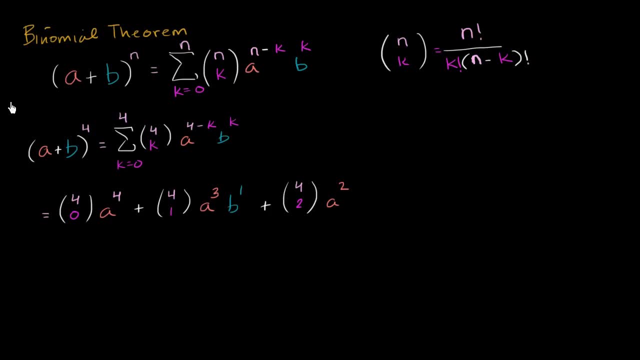 a to the fourth, a to the third, a squared, and then times b to the k. well, k is two now, so b squared, and you see a pattern again. so this is: you could say b to the zero, b to the one. 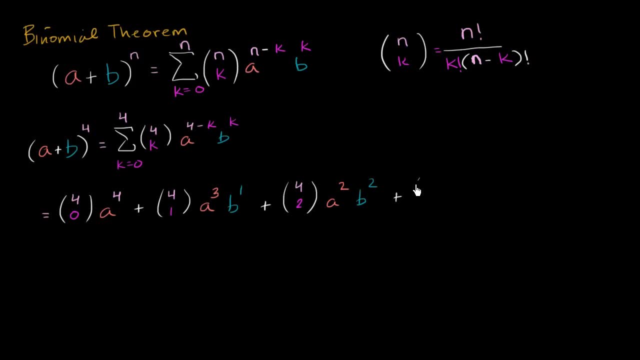 b squared, and we only have two more terms to add here: plus four, choose three, four choose three times four minus three is one times a, or a to the first, I guess we could say, and then b to the third power. 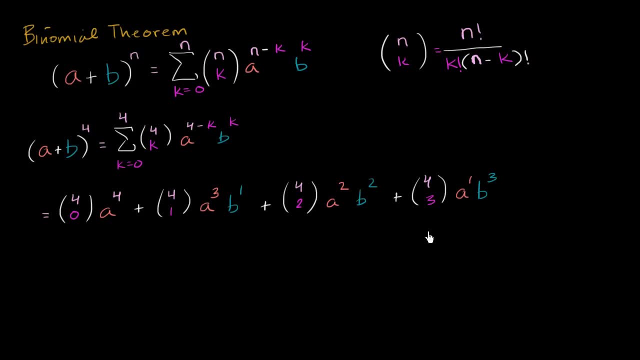 times: a to the first, b to the third, and then only one more term plus four. choose four, choose four. k is now four. this is going to be our last term. right now, we're getting k goes from zero all the way to four. 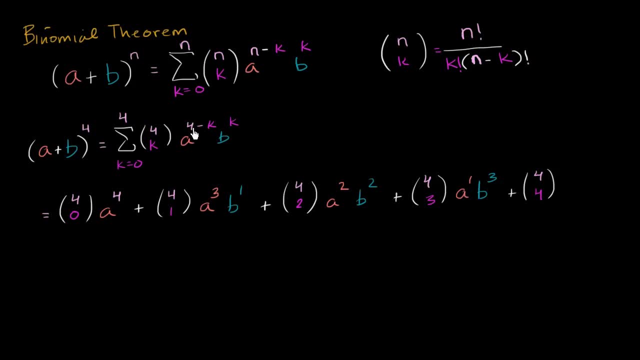 four, choose four. a to the four minus four, that's just going to be one. a to the zero, that's just one. so we're going to be left with just b to the k power, and b is four right over here. 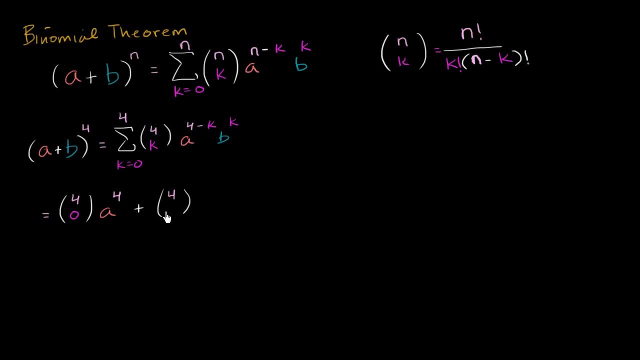 the coefficient is going to be four, choose one. and it's going to be times a to the four minus one power. so a to the third power, and I'll just stick with that color. times b to the k power. well, now, k is one. 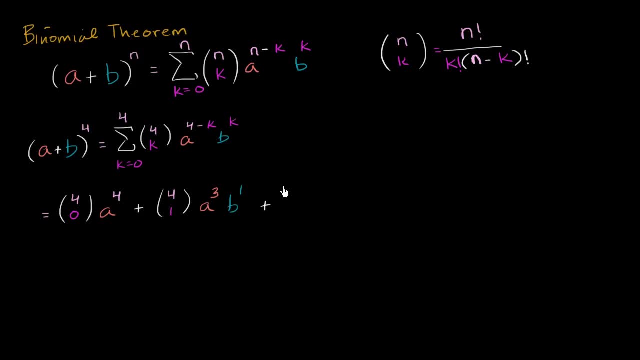 b to the first power, and then to that we're going to add, we're going to add four, choose two. four, choose two times a to the well now k is two. four minus two is two a squared. I think you see a pattern here. 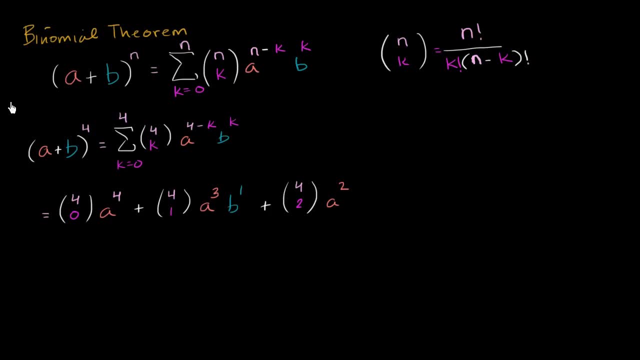 a to the fourth, a to the third, a squared, and then times b to the k. well, k is two now, so b squared, and you see a pattern again. so this is: you could say b to the zero, b to the one. 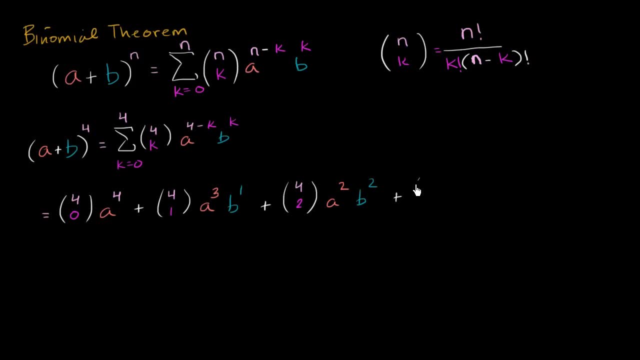 b squared, and we only have two more terms to add here: plus four, choose three, four choose three times four minus three is one times a, or a to the first, I guess we could say, and then b to the third power. 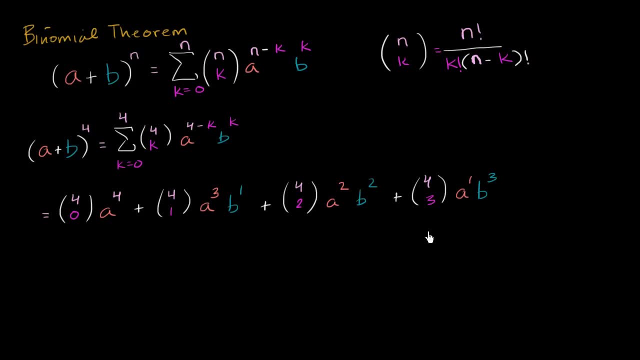 times: a to the first, b to the third, and then only one more term plus four. choose four, choose four. k is now four. this is going to be our last term. right now, we're getting k goes from zero all the way to four. 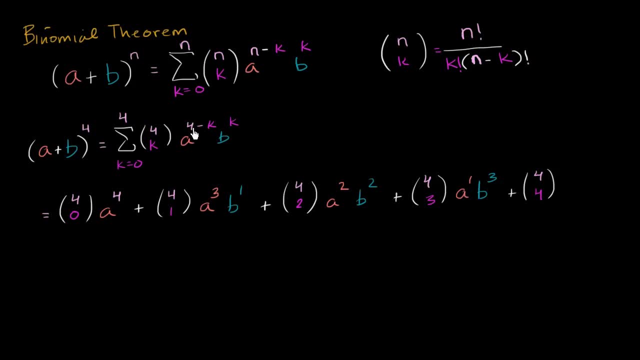 four, choose four. a to the four minus four, that's just going to be one. a to the zero, that's just one. so we're going to be left with just b to the k power, and b is four right over here. 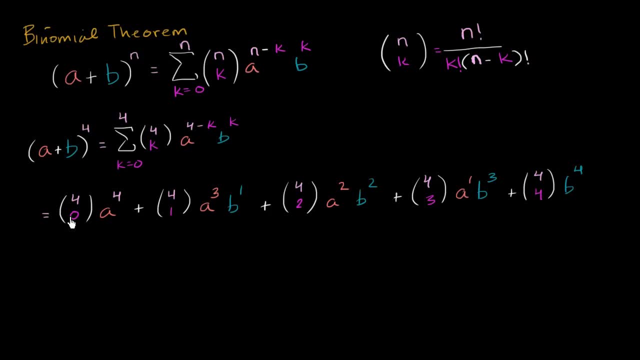 so we're almost done. we've expanded it out. we just need to figure out what four choose zero, four choose one, four choose two, et cetera, et cetera are. so let's figure that out, so we could just apply this over and over again. 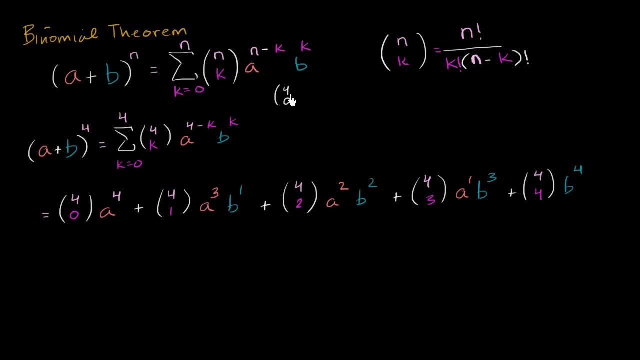 so four choose zero, four choose zero is equal to four factorial over zero factorial times four minus zero factorial. so that's just going to be four factorial, again zero factorial. at least for these purposes we are defining to be equal to one. 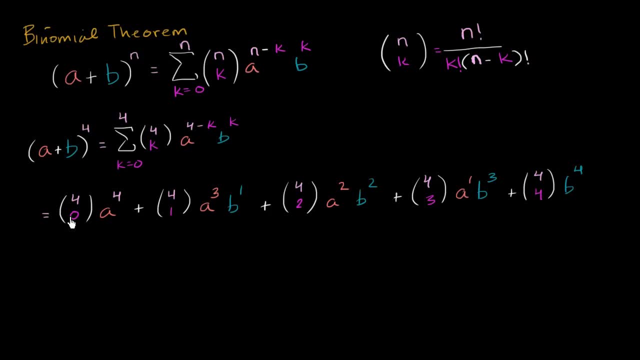 so we're almost done. we've expanded it out. we just need to figure out what four choose zero, four choose one, four choose two, et cetera, et cetera are. so let's figure that out, so we could just apply this over and over again. 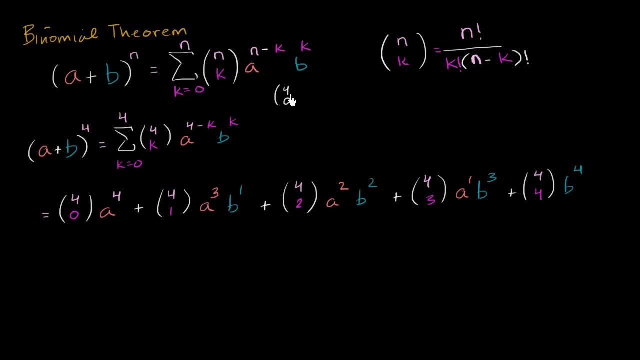 so four choose zero, four choose zero is equal to four factorial over zero factorial times four minus zero factorial. so that's just going to be four factorial, again zero factorial. at least for these purposes we are defining to be equal to one. 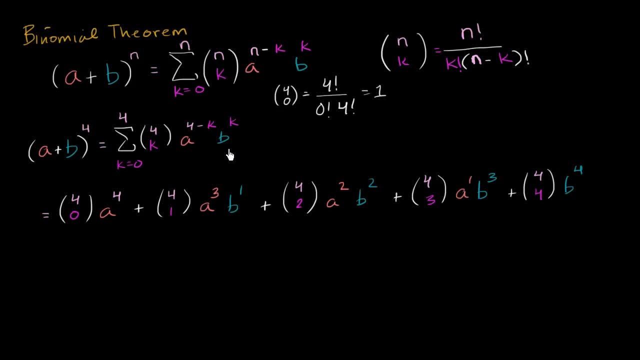 so this whole thing is going to be equal to one. so this coefficient is one. let's see, let's keep going here. so four, choose one is going to be four factorial over one factorial times four minus one factorial. four minus one factorial. 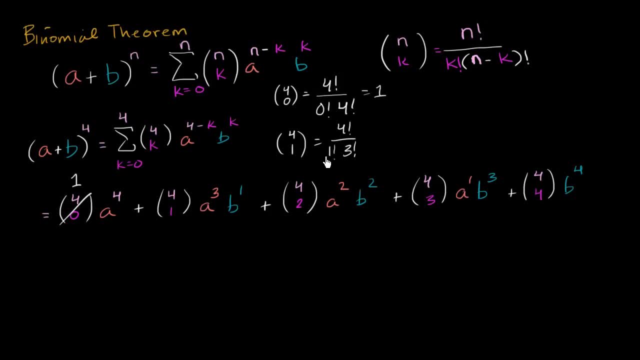 so three factorial. well, what's this going to be? well, one factorial is just going to be one. four factorial is four times three times two times one. three factorial is three times two times one. let me make that clear: four times three times two times one. 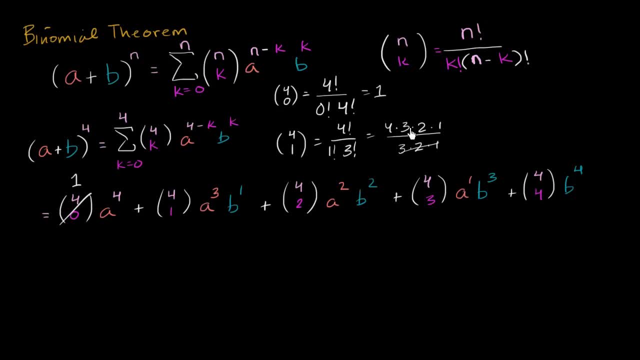 over three times two times one. it's just going to leave us with four. so this right over here is just going to be four. then we need to figure out what four choose two is. four choose two is going to be four factorial. 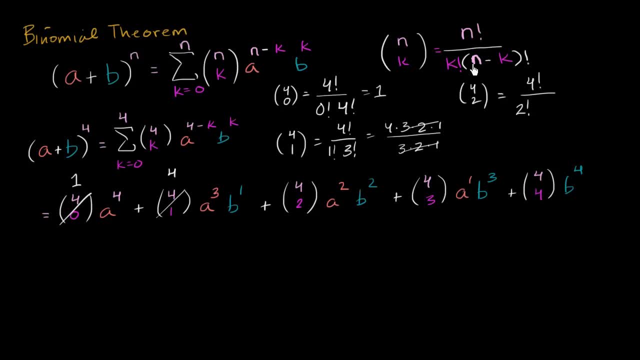 over two factorial times. what's four minus? this is going to be n minus k, four minus two over two factorial. so what is this going to be? let me scroll over to the right a little bit. so this is going to be four times three times, two times one. 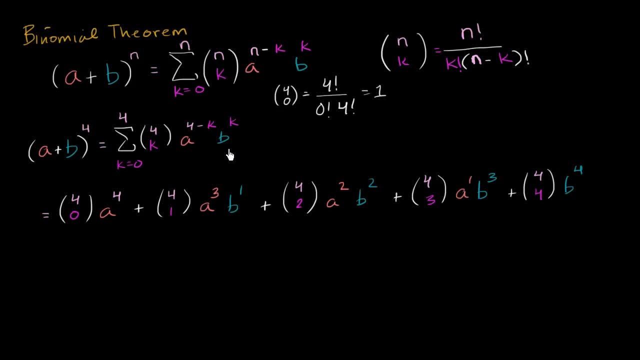 so this whole thing is going to be equal to one. so this coefficient is one. let's see, let's keep going here. so four, choose one is going to be four factorial over one factorial times four minus one factorial. four minus one factorial. 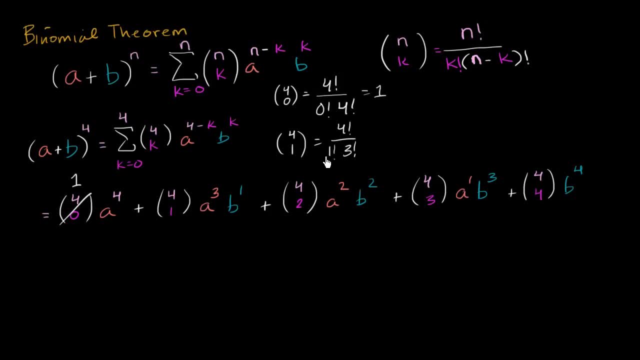 so three factorial. well, what's this going to be? well, one factorial is just going to be one. four factorial is four times three times two times one. three factorial is three times two times one. let me make that clear: four times three times two times one. 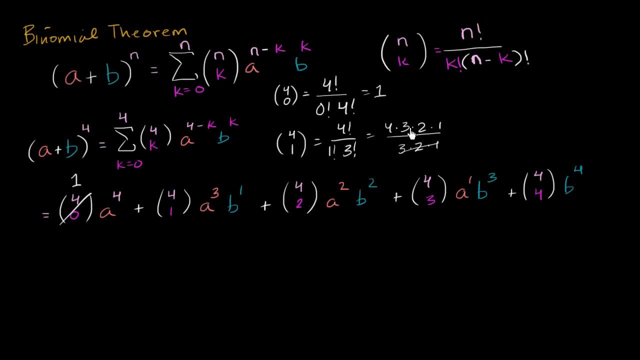 over three times two times one. it's just going to leave us with four. so this right over here is just going to be four. then we need to figure out what four choose two is. 2 is 4. choose 2 is going to be 4 factorial over 2 factorial. 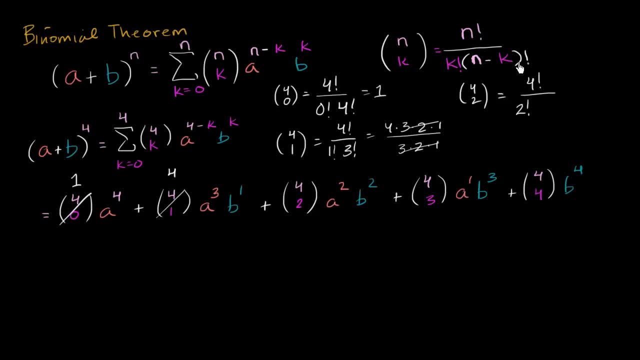 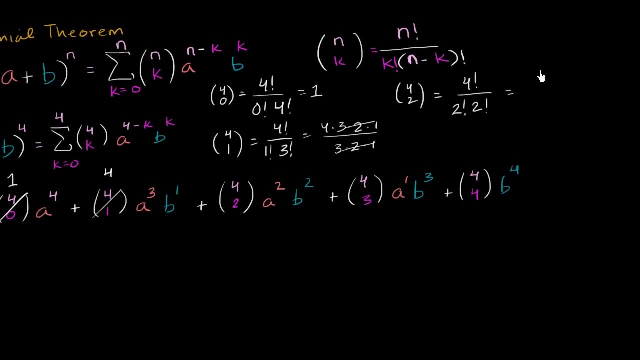 times what's 4 minus? this is going to be n minus k, 4 minus 2 over 2 factorial. So what is this going to be? Let me scroll over to the right a little bit. So this is going to be 4 times 3 times 2 times 1 over. 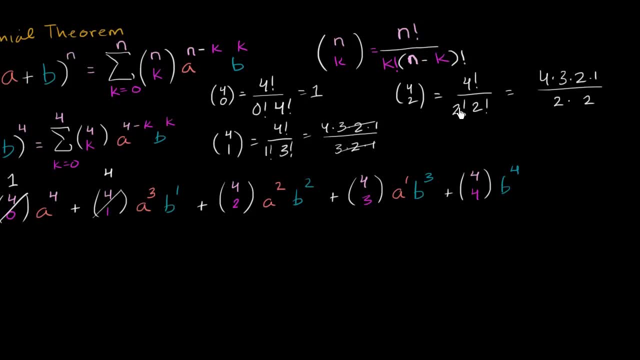 2, factorial is 2, over 2 times 2.. This is 2, this is 2.. So 2 times 2 is the same thing as 4.. We're left with 3 times 2 times 1, which is equal to 6.. 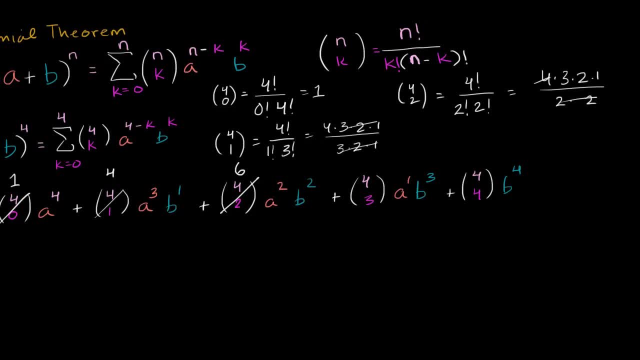 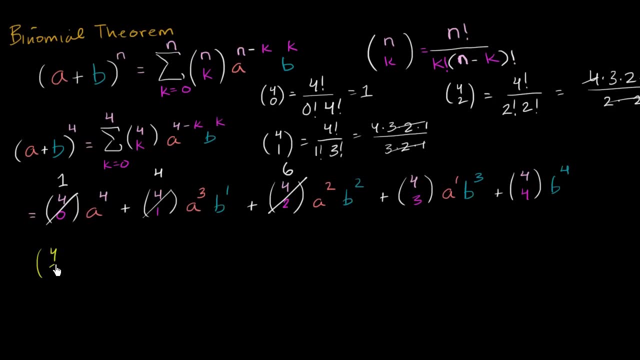 So that's equal to 6.. And then what is 4 choose 3?? Actually, I'll use some space down here. So 4 choose 3 is equal to 4 factorial over 3 factorial times 4 minus 3 factorial. 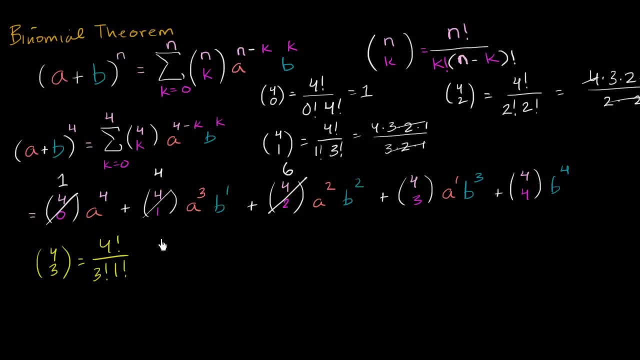 So that's just going to be 1 factorial. Well, we already figured out what that is. That's the same thing as this right over here: You just swap the 1 factorial. You just swap the 1 factorial and the 3 factorial. 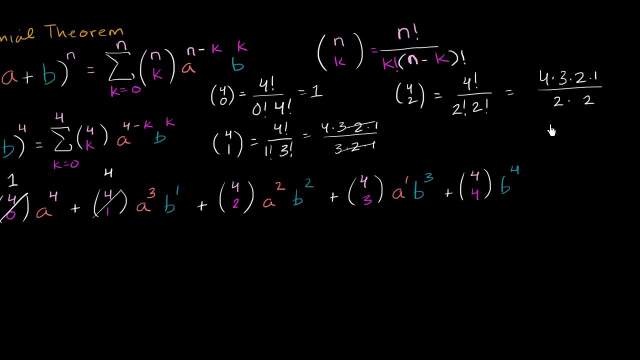 over two. factorial is two over two times two. this is two, this is two. so two times two is the same thing as four, but three times two times one, which is equal to six, so that's equal to six. 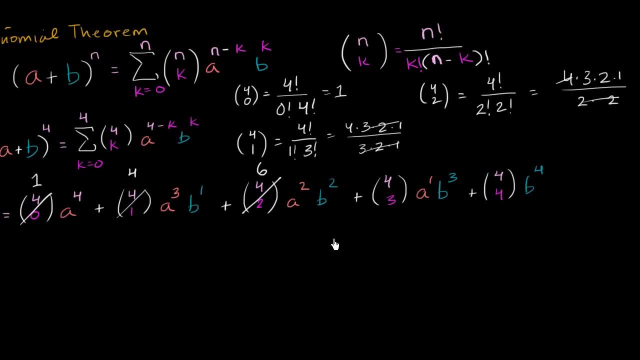 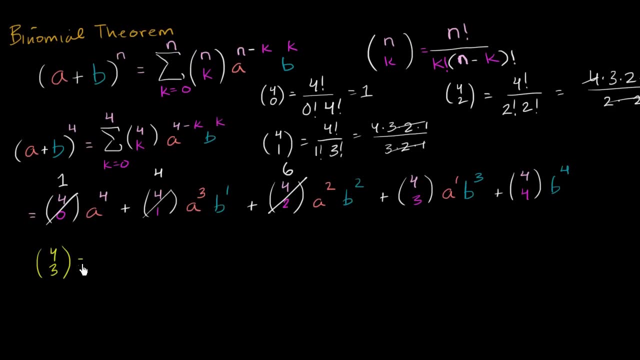 and then what is four choose three- actually I'll use some space down here- so four choose three. four choose three is equal to four factorial over over three factorial times four minus three factorial, so that's just going to be one factorial. 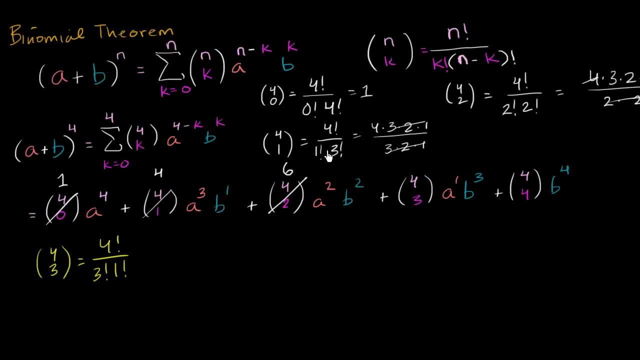 well, we already figured out what that is. that's the same thing as this right over here. we just dropped the one factorial and the three factorial, so we already figured out that this is going to be equal to four. so that is equal to four. 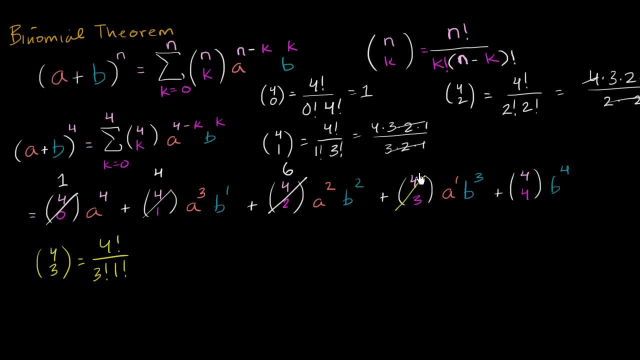 So we already figured out that this is going to be equal to 4.. So that is equal to 4.. And 4 choose 4?? Well, this is just going to be. let me just do it over here: 4 choose 4 is 4 factorial over 4 factorial times 0 factorial. 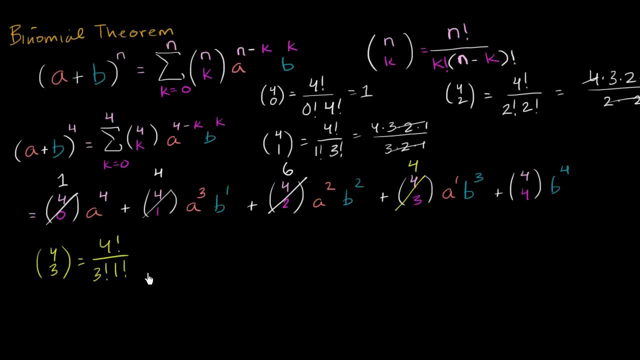 and four choose four. well, this is just going to be. let me just do it over here: four choose four is four factorial over four factorial times, zero factorial, which is the exact thing we had here, which we figured out was one. 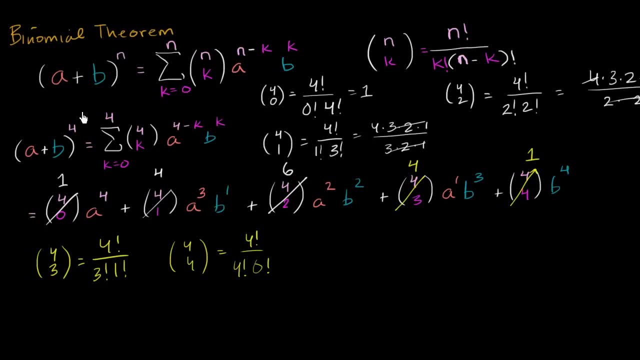 and just like that we're done. we were able to figure out what a plus b to the fourth power is. it's one a to the fourth plus four, a to the third, b to the first plus six. a squared, b squared. 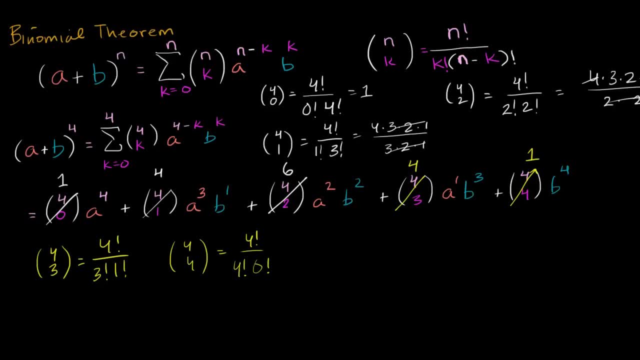 plus four, a cubed plus b to the fourth, and actually let me just write that down, since we did all that work. this is equal to a to the fourth plus plus four plus four. a to the third, a to the third b. 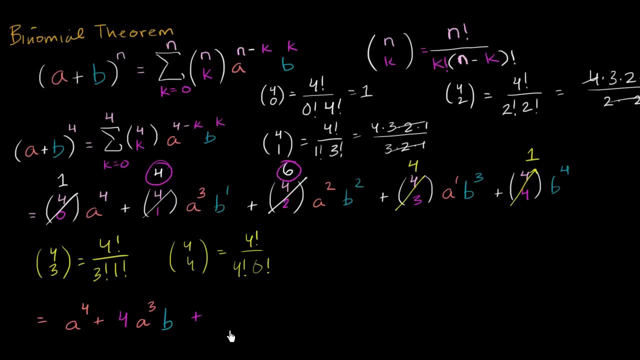 plus plus six plus six: a squared, b squared, a squared b squared. plus plus plus four. I think you see a pattern here: plus four, a a times b to the third power, plus b to the fourth power. 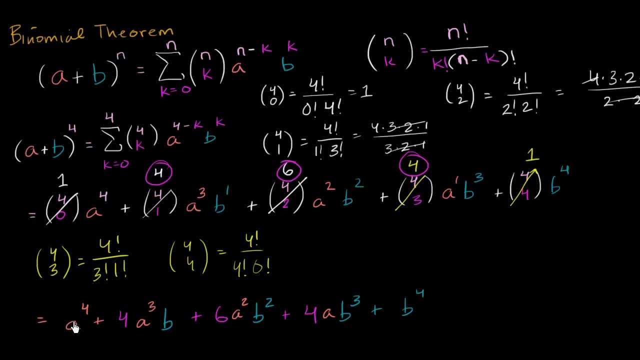 plus b to the fourth power. and there's an interesting pattern here. there's a symmetry where you have the coefficient, you go one, four, six and for the middle term, and then you go back to four and then you go back to one. 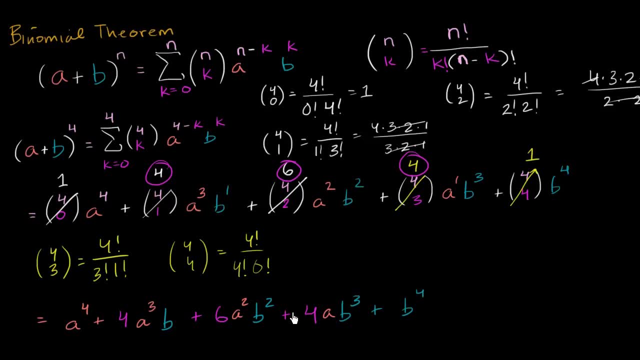 and then you also see, that pattern is that you start at a to the fourth, a to the third, a squared a, and then you could say there's an a to the zero here, and then you start at b to the zero. 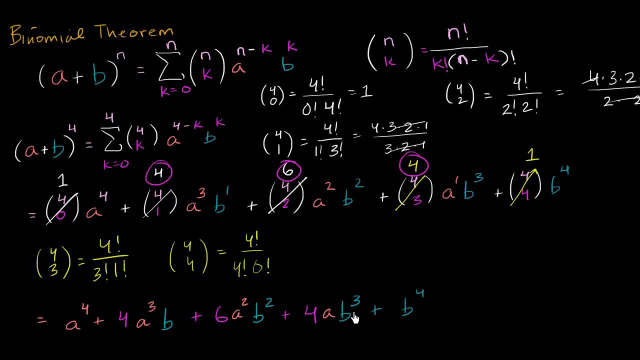 we didn't write it, but that's just one. then b to the first, b squared, b to the third, b to the fourth. so this is just one application, or one example. in future videos we'll do more examples of the binomial theorem.